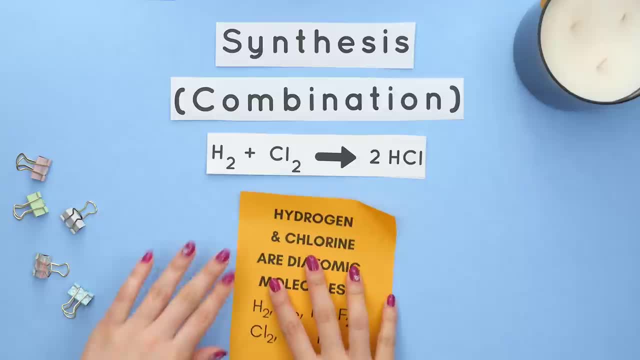 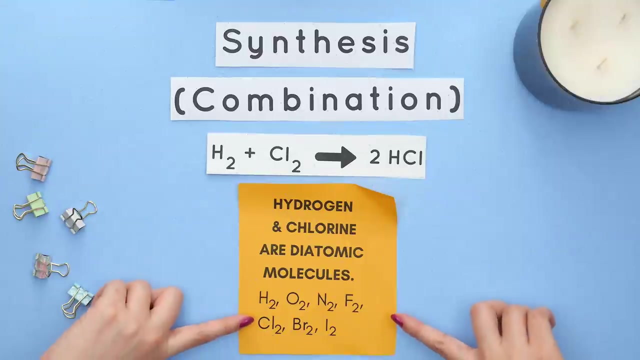 reactants combine to form our product. Note: the reason why hydrogen and chlorine have a two subscript is because they are known as being diatomic molecules. Diatomic molecules are atoms that exist in pairs. Here is a list of diatomic molecules. Now, if we flip this, 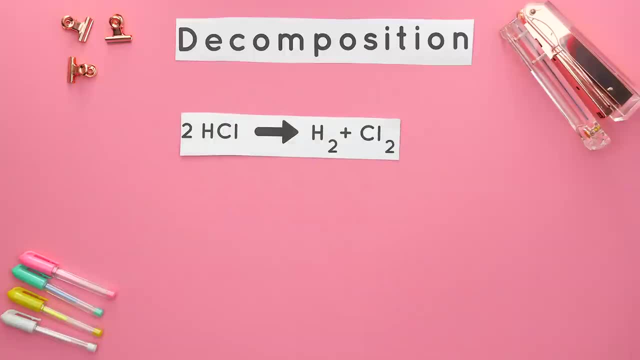 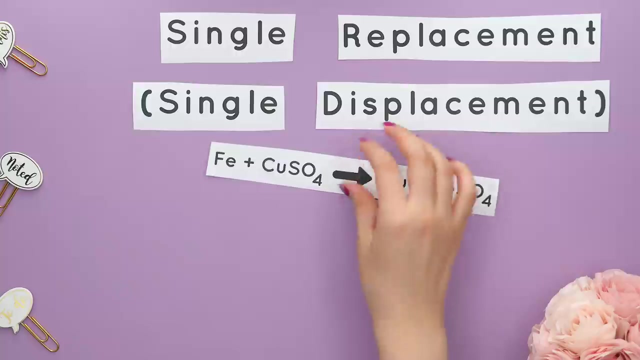 synthesis reaction. you'll see it's now a decomposition reaction, Because in a decomposition reaction you have one reactant that is being broken apart into multiple products. The next reaction is a single replacement or a single displacement reaction. Here's an example: Our reactants are one element plus one compound and those form one element plus. 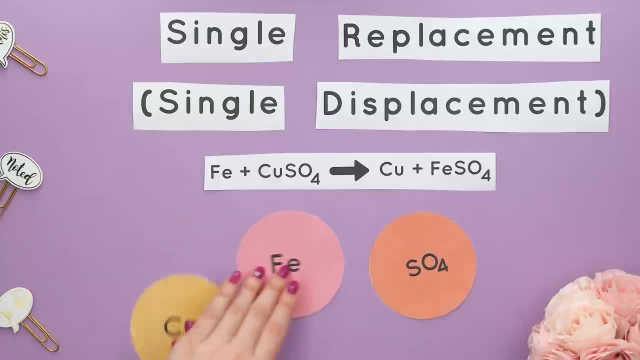 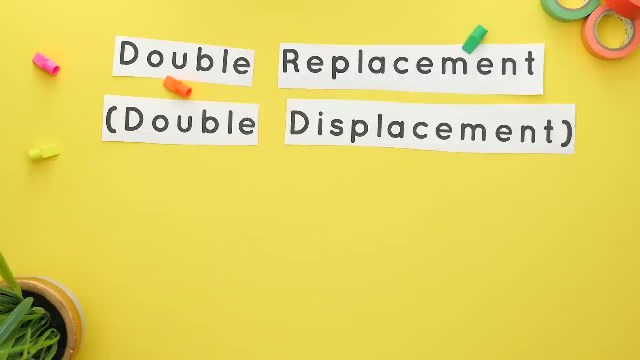 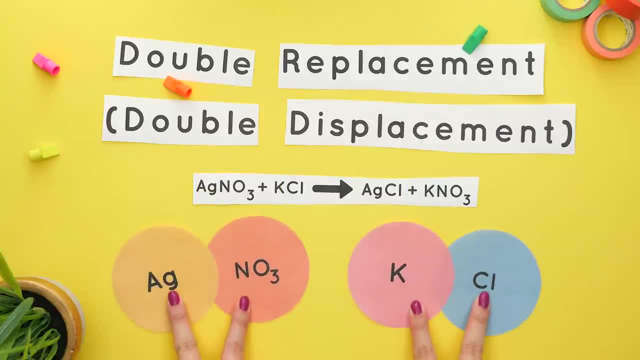 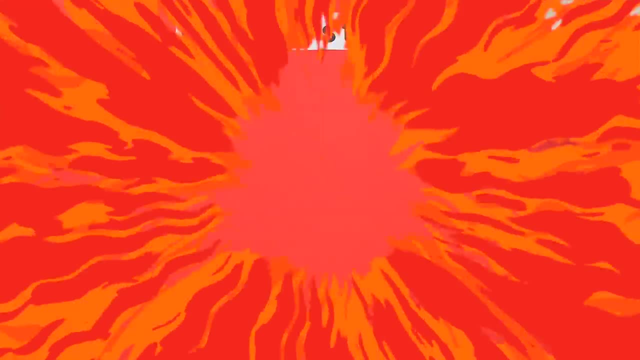 elements combine and the outer elements combine, and the outer elements combine and the outer elements combine to form our new products. Or you can think of it as the metals are switching again to form our new products. Up next is a combustion reaction, which occurs when something is burning. This is the general equation. 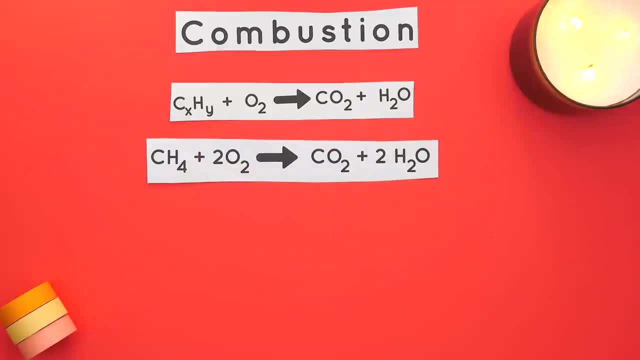 and here's our example where our first reactant consists of only carbon and hydrogen. Or we can have our first reactant consisting of carbon, hydrogen and oxygen. Your biggest clue that something is a combustion reaction is that the second reactant is O2, and our products are. 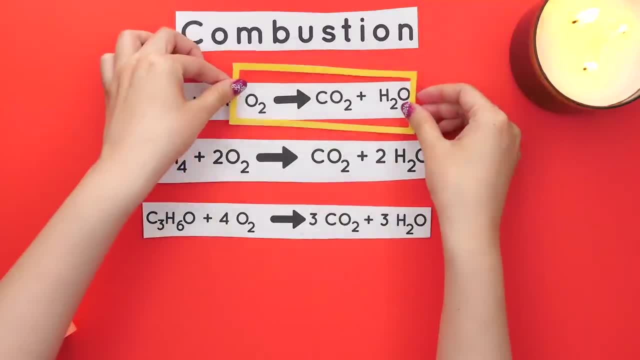 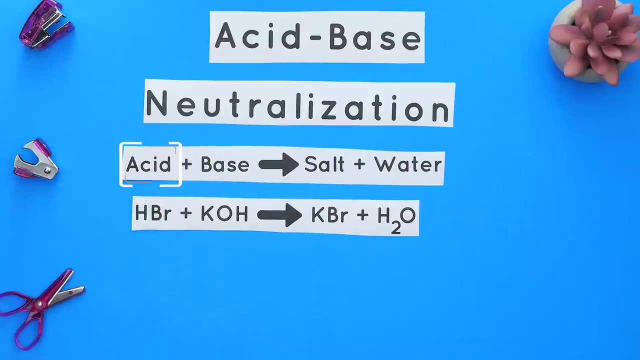 carbon dioxide and water. These never, ever change. Now, in an acid-base neutralization reaction, we have an acid plus a base, and those form a salt and water. Now, if you're unsure what an acid base or salt looks like, an acid typically starts with an H or hydrogen. 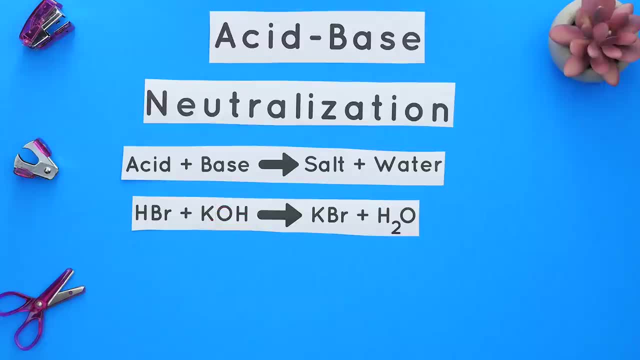 And a base will end with OH or hydroxide, And a salt is a type of ionic compound which consists of a metal and a non-metal which have opposite charges. Predicting products is the next thing you're going to need to know.